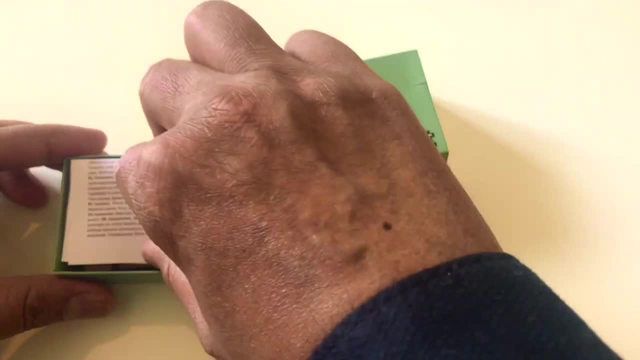 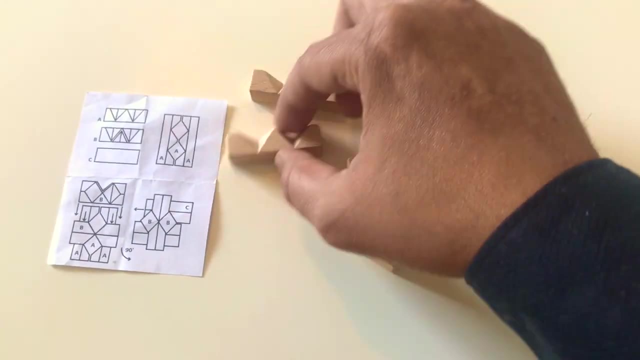 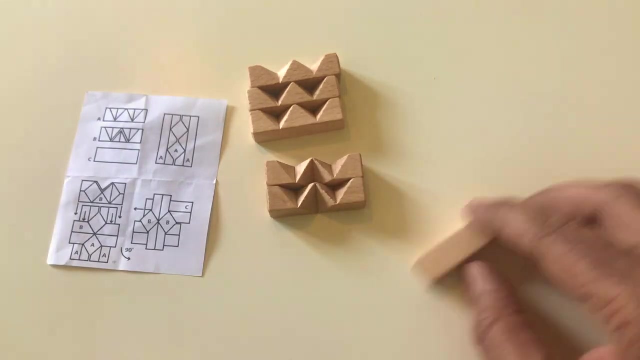 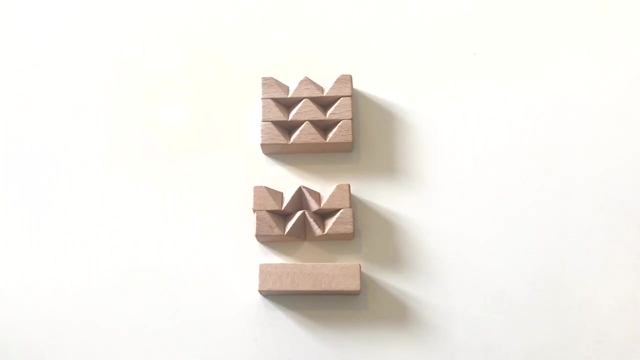 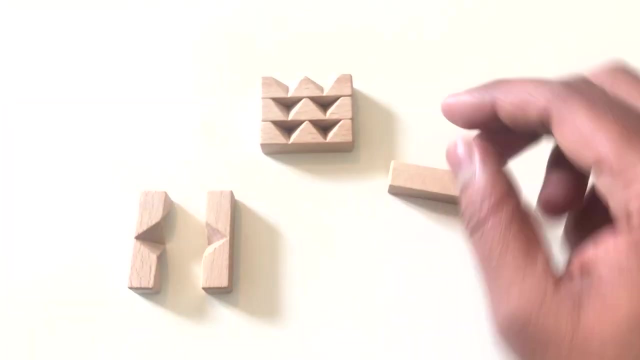 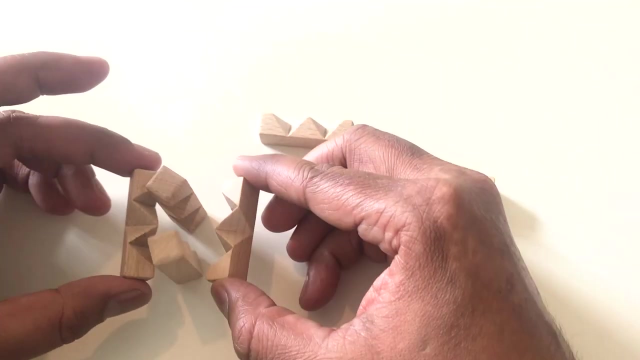 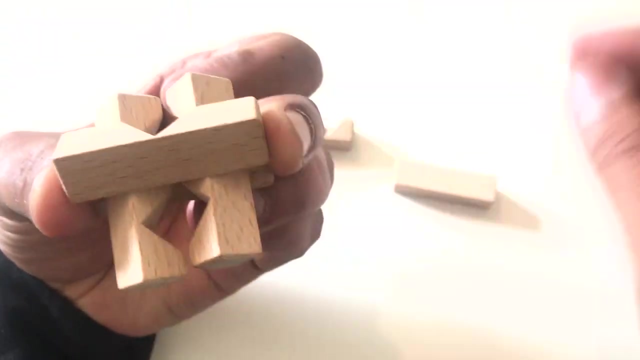 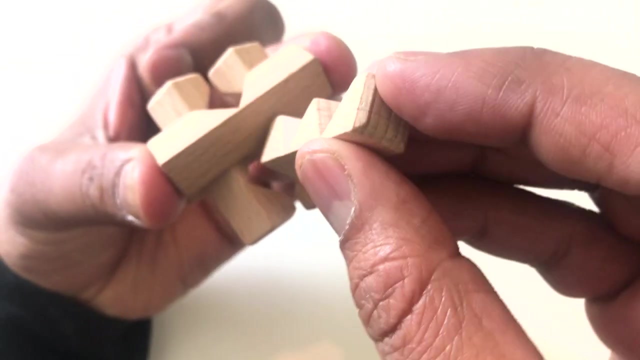 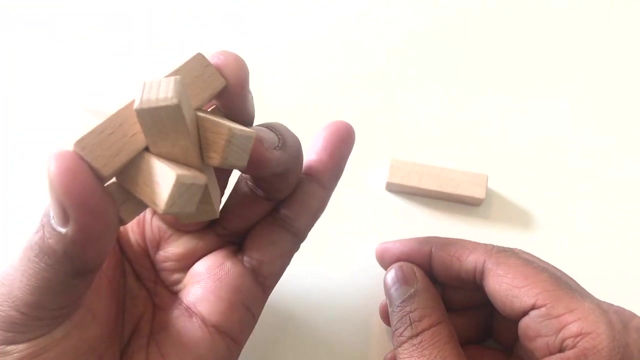 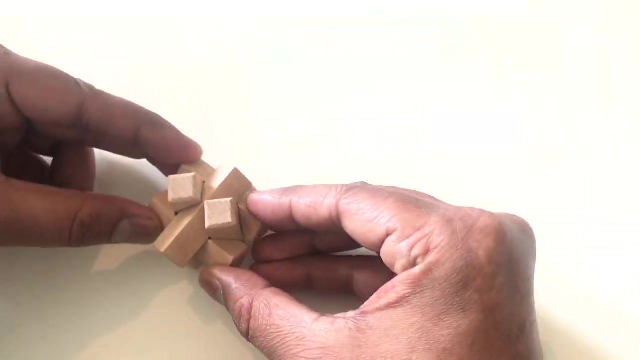 This video is a derivative work of the project. Please select a language. Thank you, Thank you. 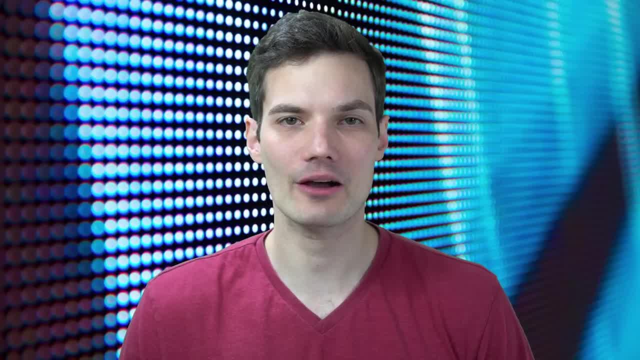 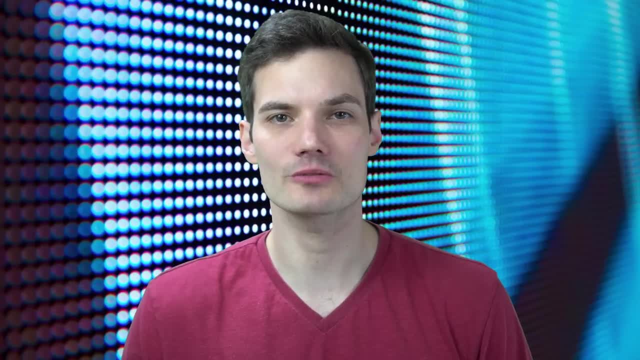 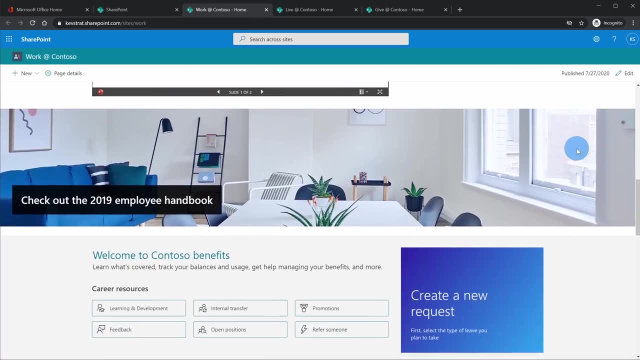 Hi everyone. Kevin, here Today I want to show you how you can use Microsoft SharePoint. First off, what is Microsoft SharePoint? It's a place you go to work with others and also to stay informed. Okay, but what does that actually mean and what can you do with SharePoint? 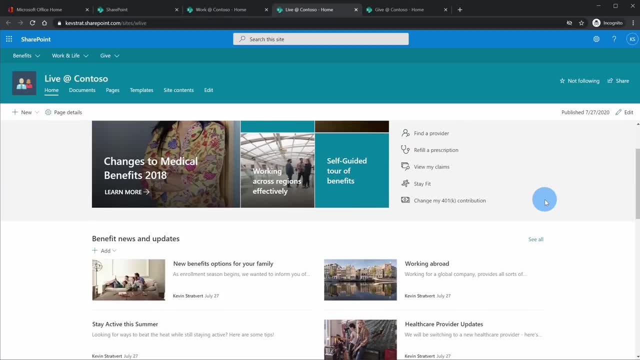 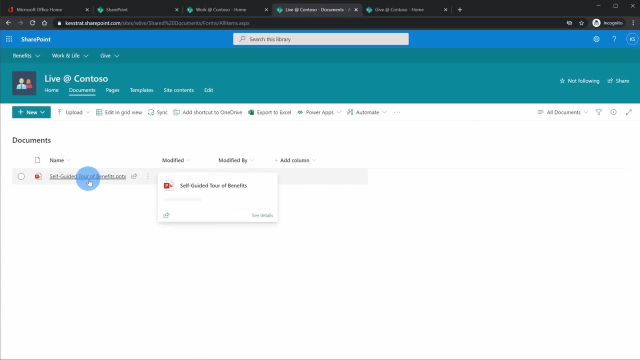 With SharePoint, you can set up an intranet site for your team, basically a webpage for your team, and you could customize it without needing to know any coding. You could set up a document repository so you can upload a file to your SharePoint site, and then everyone. 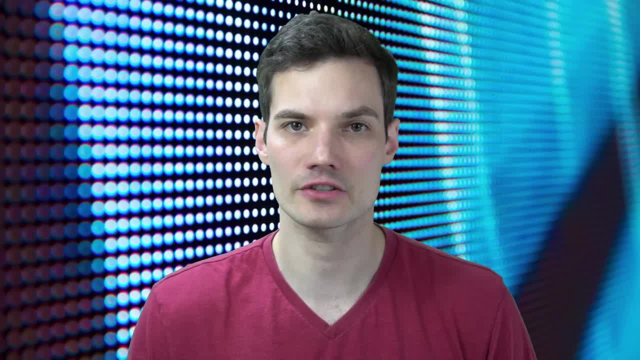 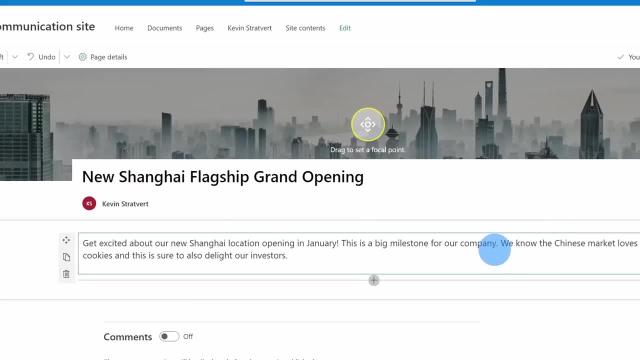 on your team will have access to that file. You could have shared calendars, You could create lists and everyone can contribute to that list, and you could also publish news posts to keep your entire team informed. It does quite a bit. There are two different. 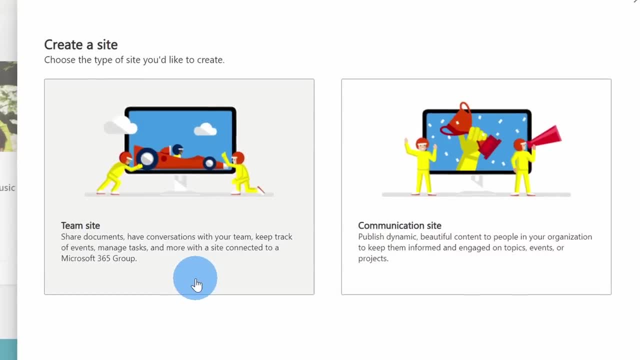 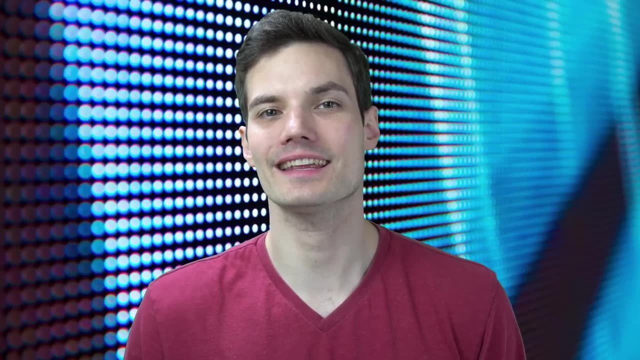 types of SharePoint sites. You have team sites and also communication sites, and we'll walk through what some of those differences are. All right, why don't we jump on the PC and, first off, let's look at what is a SharePoint site. Let's look at how we can get SharePoint. To be able to get SharePoint, you need either: